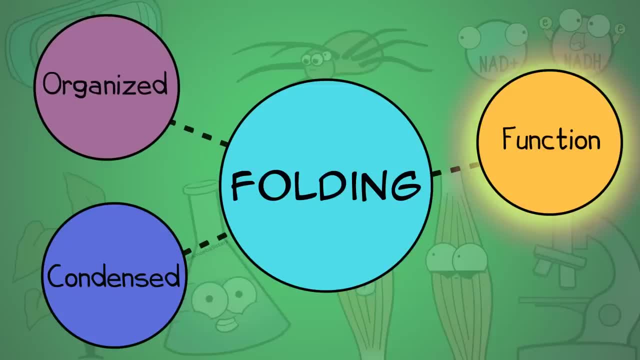 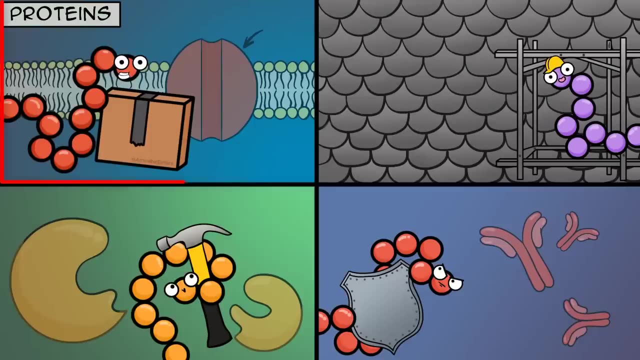 This is true, But in biology, folding can actually have a lot to do with function. We've mentioned how amazing proteins are. They can play so many roles. They can make up channels, be part of a structure, serve as enzymes for important biological processes, be involved. 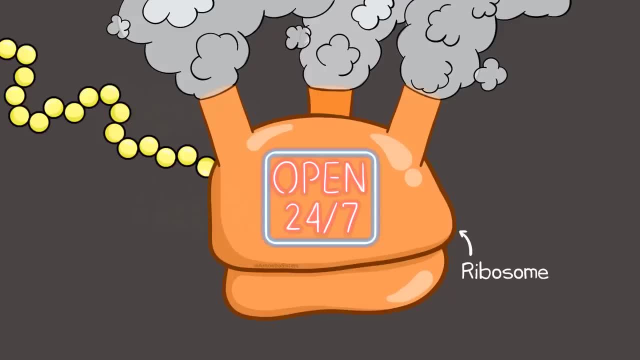 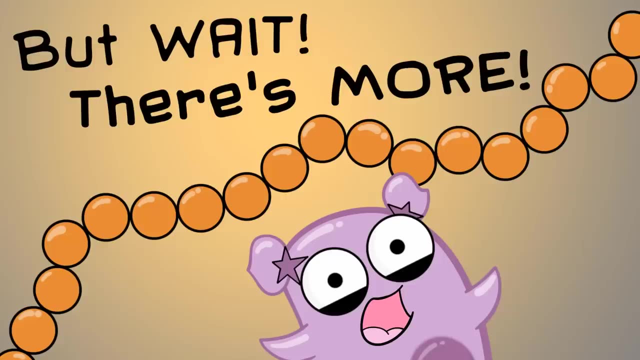 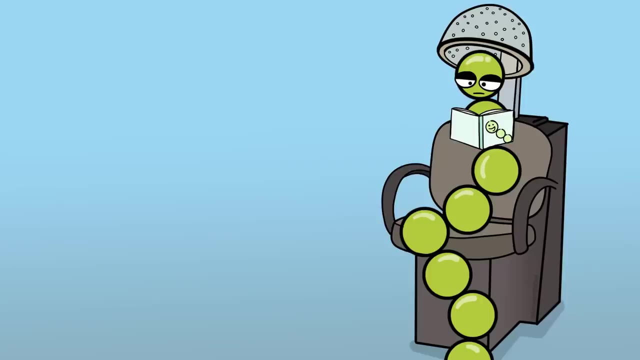 with protecting the body, just to name a few. We've also mentioned that you are making proteins all the time in a process known as protein synthesis, But the conclusion of producing a long chain of amino acids doesn't necessarily equal a functional protein. There are modifications to a protein that often need to happen in. 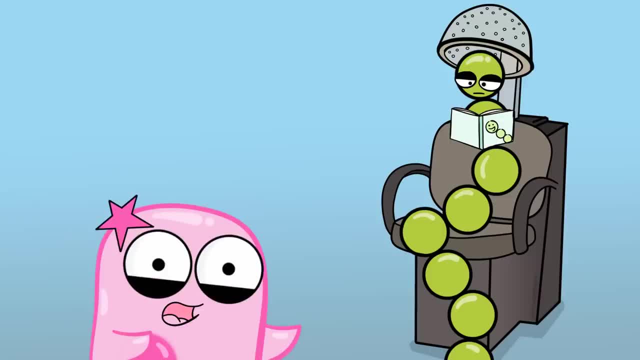 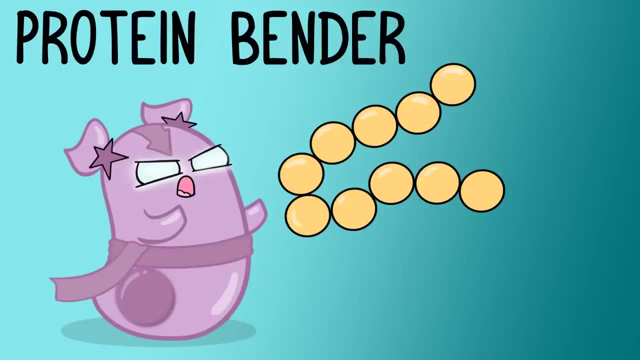 order for it to be functional. By modifications we can mean many things. It might be adding certain chemical groups, such as phosphorylation- something to definitely explore- But another important event to make a functional protein is, believe it or not, folding. 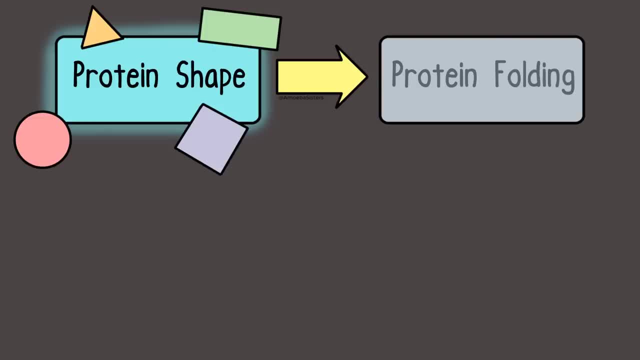 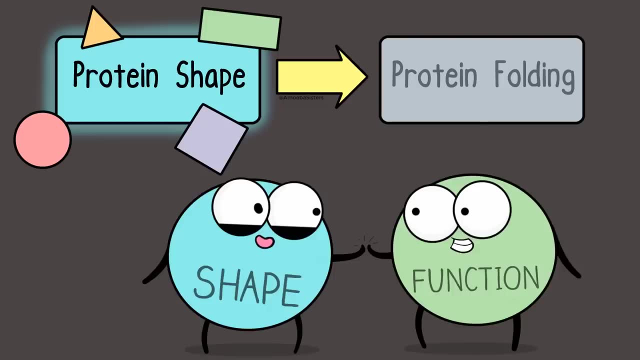 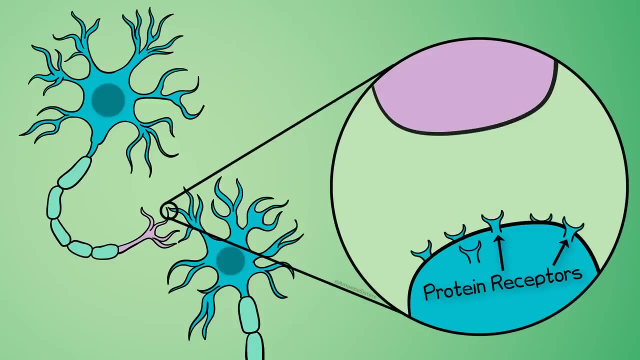 But before we get into protein folding, let's talk about shape and why shape is so important. Shape and function in biology frequently go hand in hand. In our cell signaling video we mention how protein receptors and the signal molecules that bind them can fit together so perfectly to start some type of cellular response. 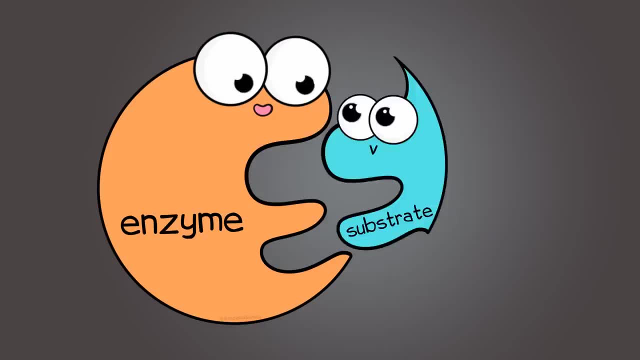 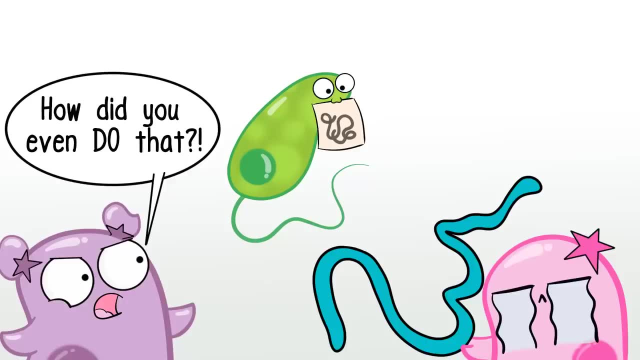 Or in our enzyme video, we talk about how enzymes, which are frequently proteins, have a very specific shape for the substrates that they build up or break down. When we talk about the way proteins are folded, we need to understand the different levels. 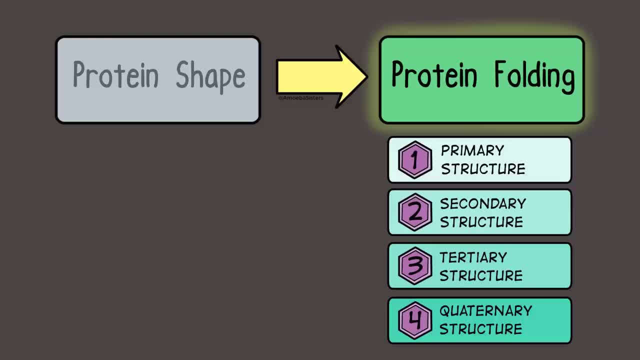 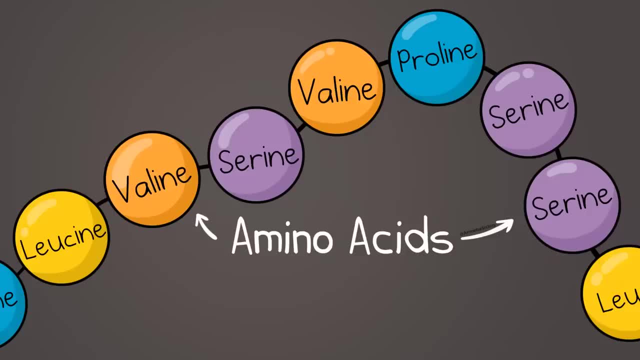 of protein structure because there are different ways of folding that can happen in the different structural levels. The first level of protein structure is primary structure. This is the sequence of amino acids that make up a protein. Amino acids are the monomer of a protein. 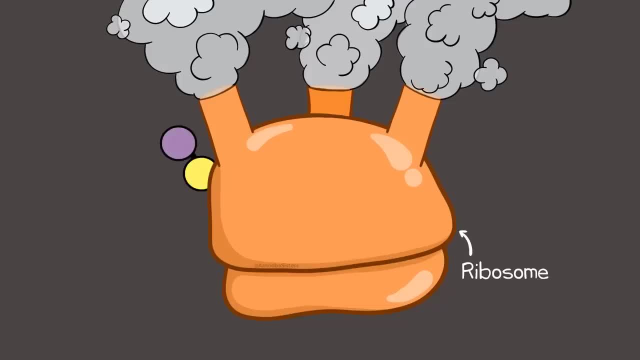 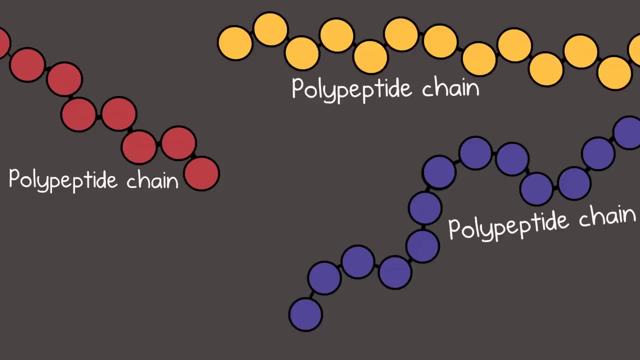 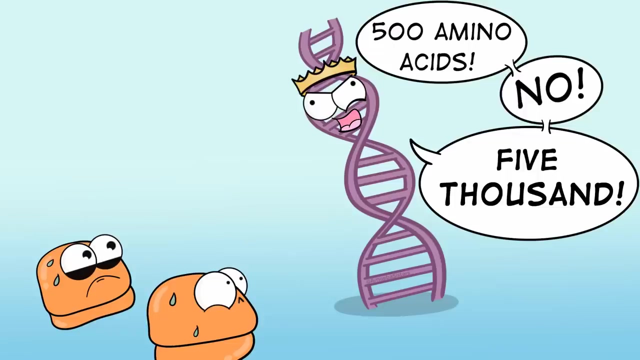 They are held together by peptide bonds. In protein synthesis, amino acids are added to form a polymer. They form a polypeptide chain and proteins are made of one or more of these polypeptide chains. Genes, which are made of DNA, determine the order and number of these amino acids. 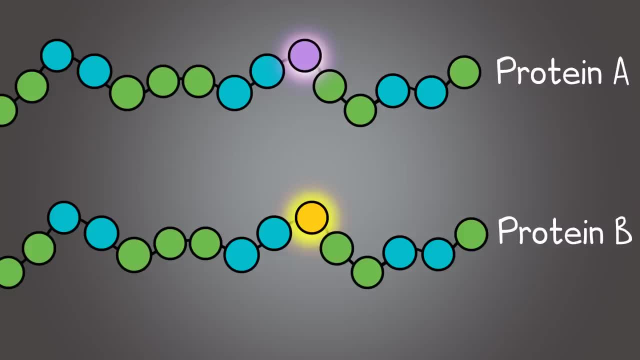 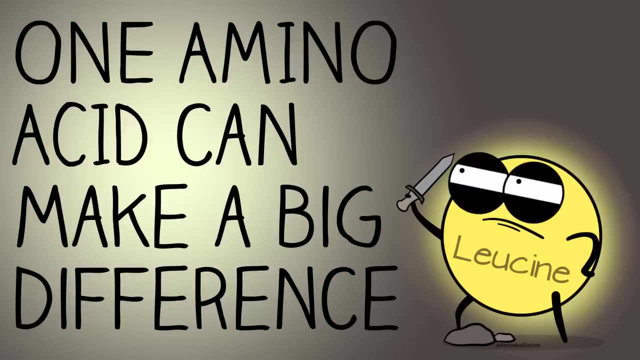 That sequence is critical to the protein's structure and function. In our mutations video we talk about how one amino acid can be changed in sickle cell disease. Even a single change of an amino acid has the potential to affect a protein's function. 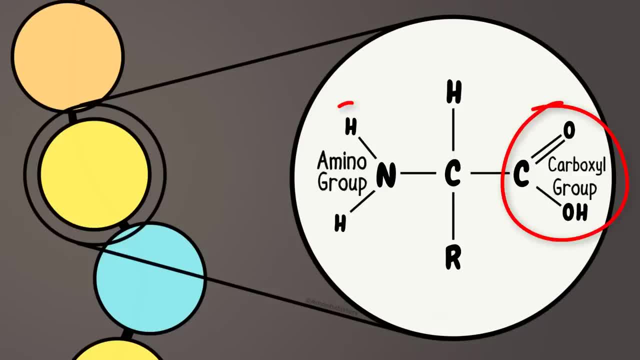 We do want to point out that each amino acid has a carboxylase. Each amino acid has a carboxyl group, an amino group and an R group. R group is also called a side chain. So, even though we have them drawn here like a chain of circles, realize that each of these 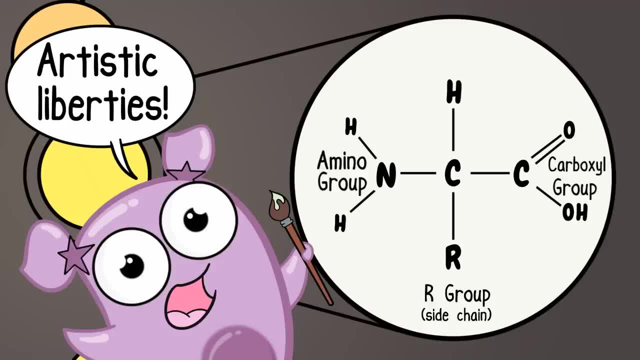 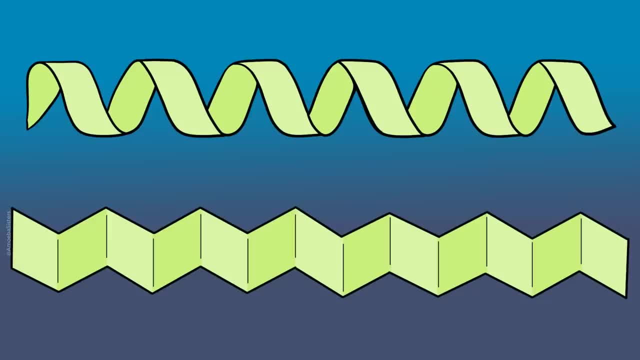 circles we're drawing is an amino acid like this. Next we move on to secondary structure. Folding is really going to start to happen In secondary structure. the sequence of amino acids that we mentioned in primary structure can fold in different ways. The most common ways are the alpha helix and the beta pleated sheet. 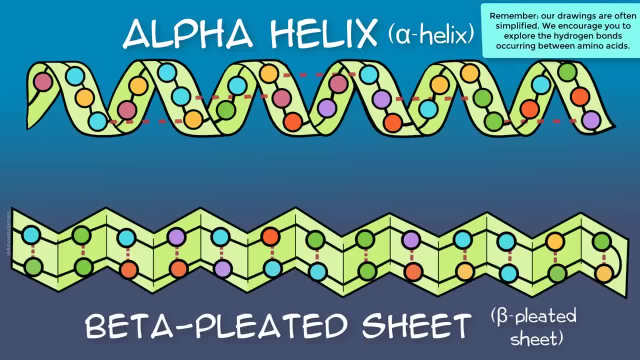 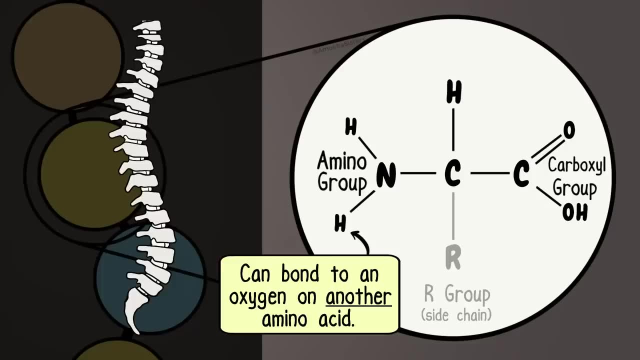 And which one of those foldings the protein does depends on the amino acid arrangement it has. Both of these shapes are due, largely in part, to hydrogen bonds. Those hydrogen bonds can occur at specific areas of the protein's amino acids. Specifically, these are hydrogen bonds involving the backbone of the amino acid structure. 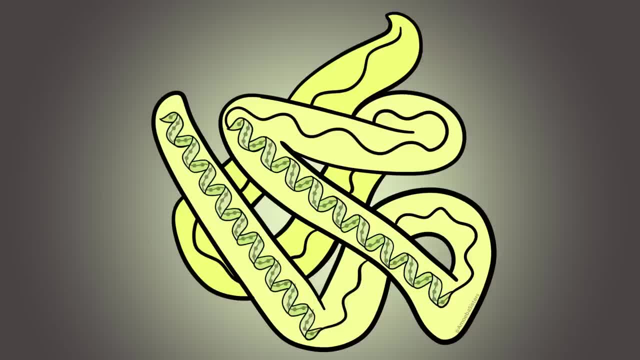 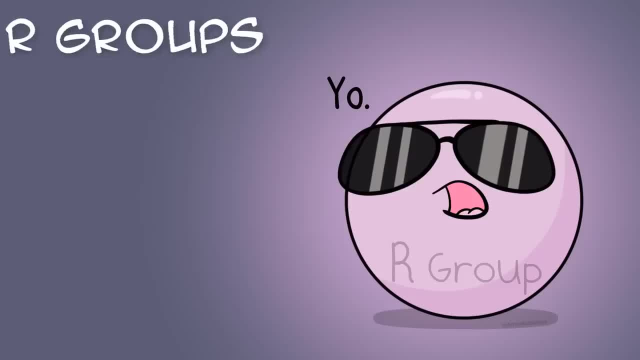 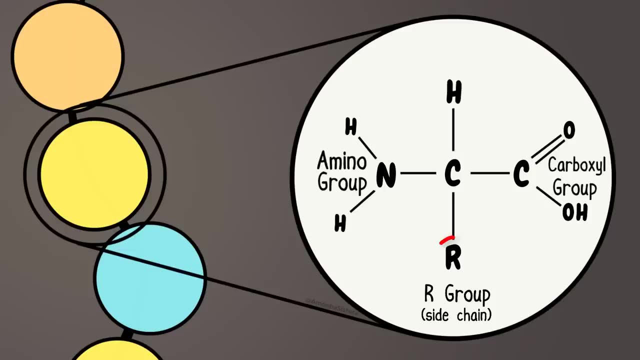 On to tertiary structure. This is looking at more folding that occurs in the 3D shape of a functional protein, And a lot of this is due to something we haven't mentioned much: The R groups, Also called side chains, See the amino group and the carboxyl group, are generally standard parts of an amino acid. 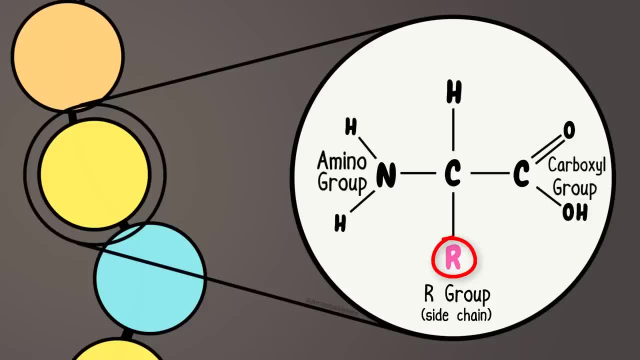 although the R group found in amino acids can vary among different amino acids, That means the R group can define the amino acid and can make amino acids behave a certain way. For example, some R groups are hydrophilic: they like water. 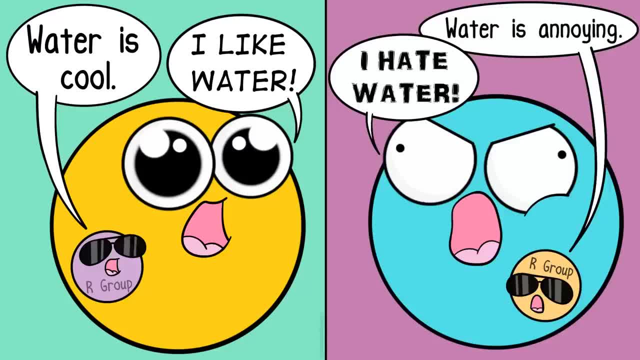 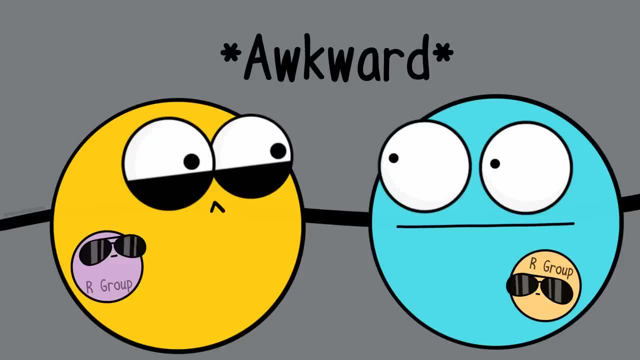 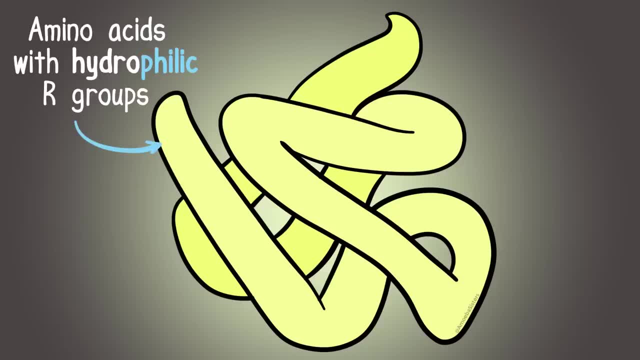 Some R groups are hydrophobic. they don't And remember that proteins contain many amino acids which can contain different R groups, and so different areas of the protein can therefore be impacted based on those R groups. When protein folding is going on, amino acids with hydrophilic R groups may hang out on the 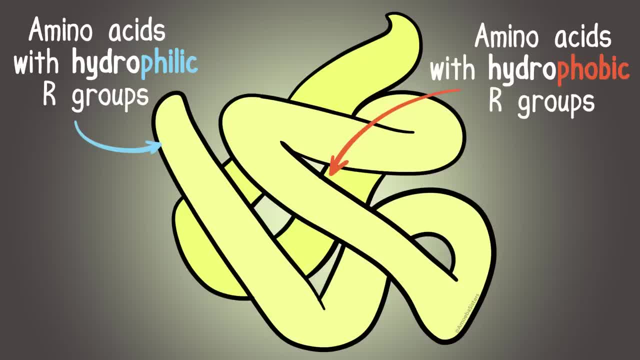 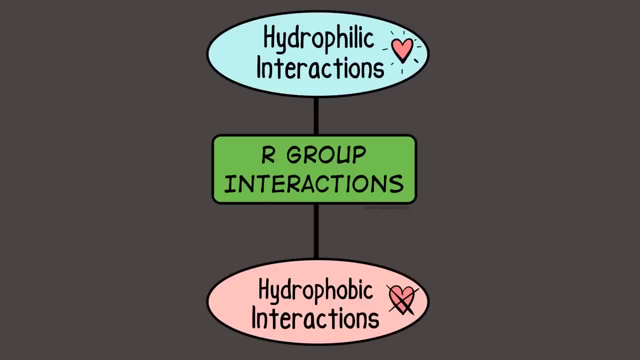 outside, while hydrophobic R groups where are they? They might hang out at the inside part of the protein. The 3D shape is due to other interactions besides hydrophobic interactions: Ionic bonds, van der Waals interactions, disulfide bonds and hydrogen bonds, all involving the 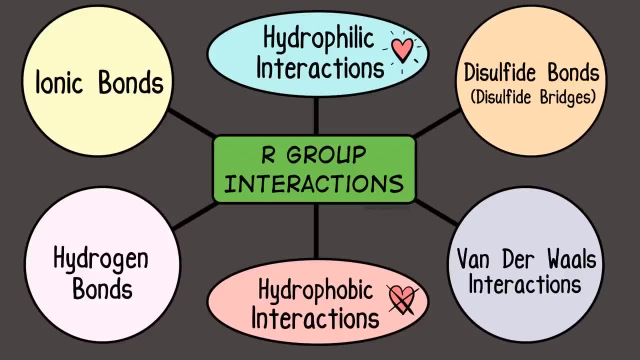 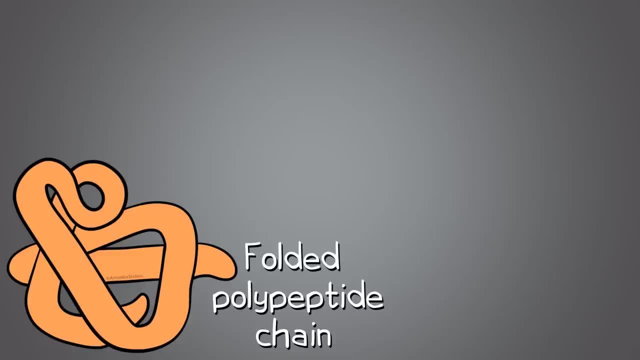 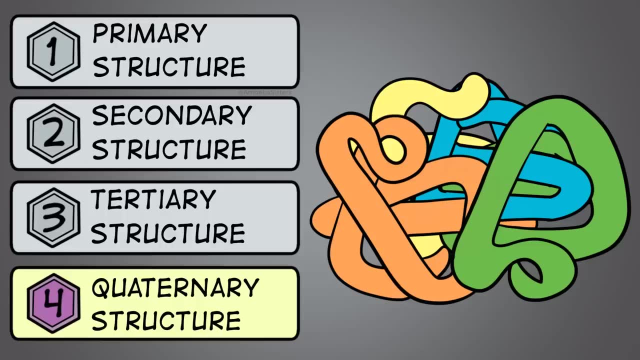 R groups. These interactions can influence the folding occurring in tertiary structure, something to explore Now. when we've been talking about a protein, we've been talking about a polypeptide chain that has been folded into a functional protein, But proteins can be made of one or more polypeptide chains and in quaternary structure you are. 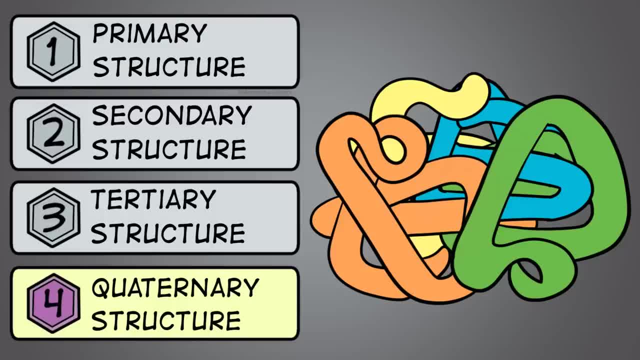 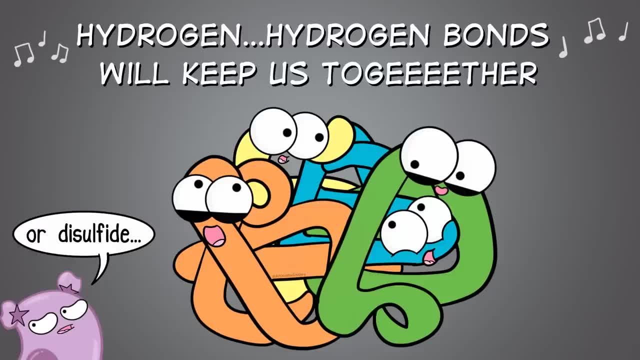 looking at a protein consisting of more than one polypeptide chain. Each of these polypeptide chains can be a subunit and interactions between them, such as hydrogen bonds or disulfide bonds, can keep them together. Going back to folding, I know what you might be thinking. 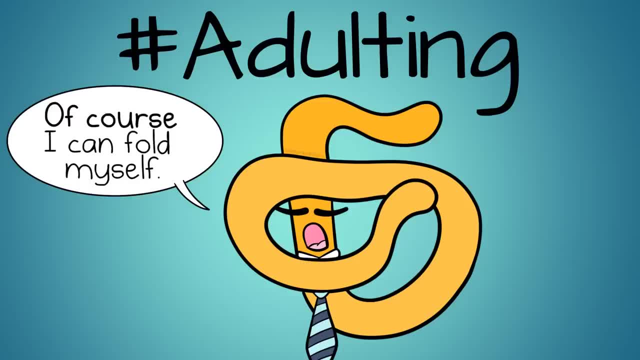 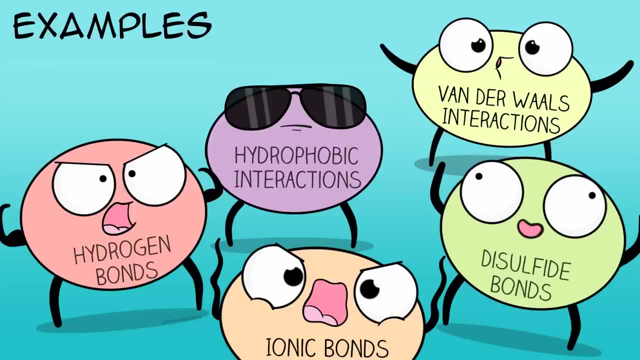 Who is doing this folding anyway? Are the proteins just folding themselves? Well, the interactions mentioned, like hydrogen bonds and R group interactions, are occurring depending on the protein's own amino acids, one reason why amino acid sequences are very important for protein function. 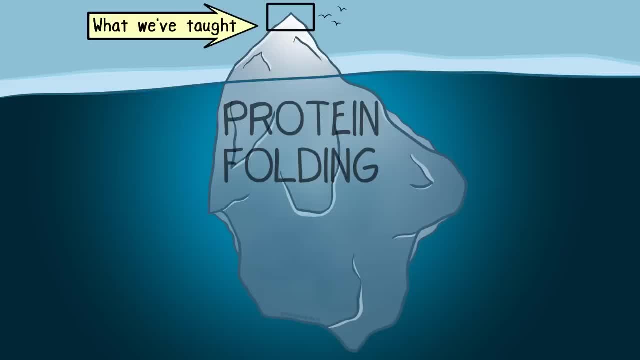 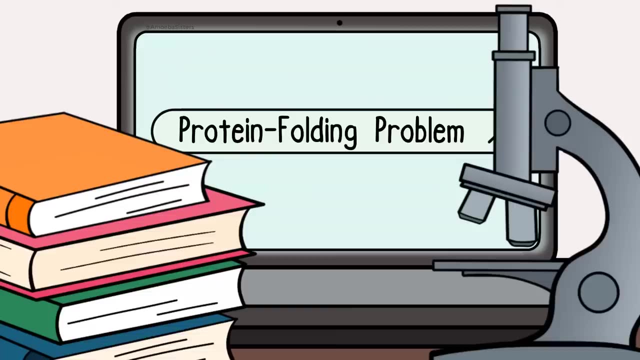 But folding is far more complex than that and there can be intermediate steps involved when a protein is folding. In fact, there's a phrase you can search called the protein folding problem, To learn more about the question scientists continue to explore regarding protein folding. 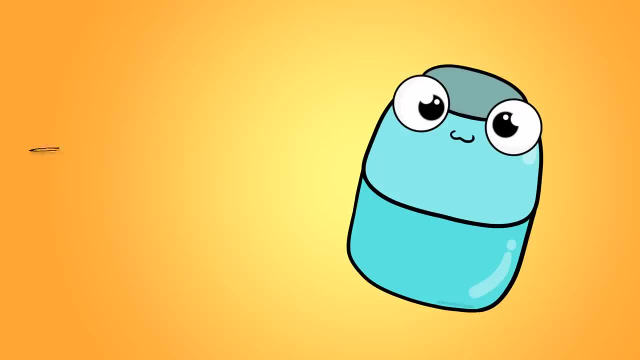 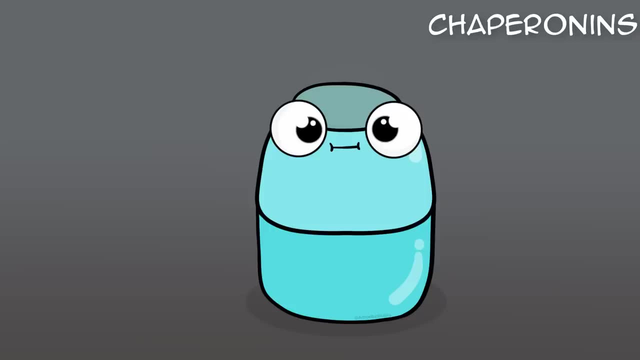 Research has shown that proteins often have help in the folding process. Chaperonins, for example, are proteins that can help with the folding process. They have almost a barrel shape, Proteins go into them and the chaperonin tends to have an environment that is ideal. 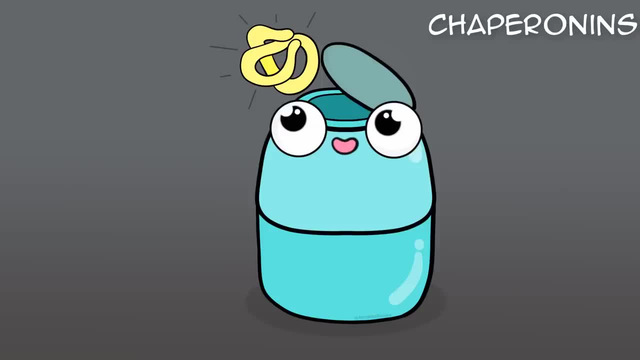 for the protein's folding And this can help the protein be folded correctly, so it's functional. Just wish I had something like that for my towels. All of these interactions we mentioned in primary, secondary and secondary are all related to the protein folding process. 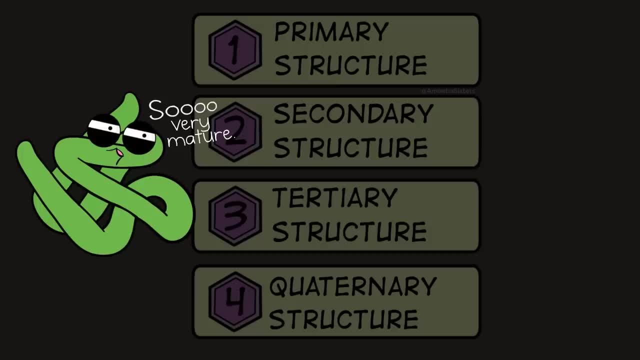 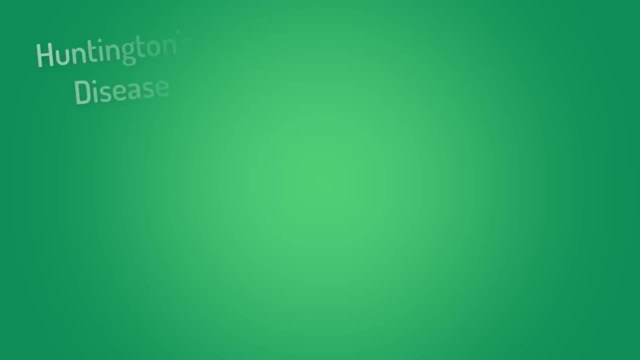 So let's get started. Primary, tertiary and quaternary structure are paramount for a mature protein to have its correct shape so it can carry out its function, And that's very relevant. There are many diseases that are related to protein misfoldings. 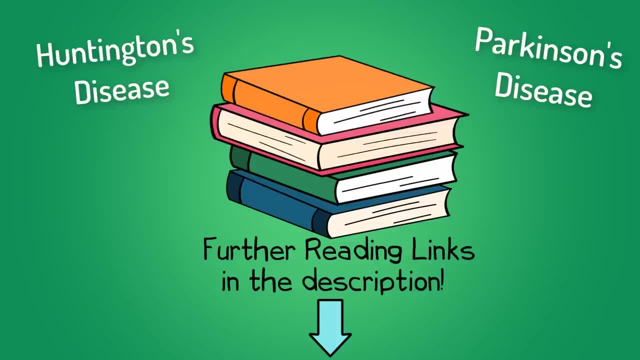 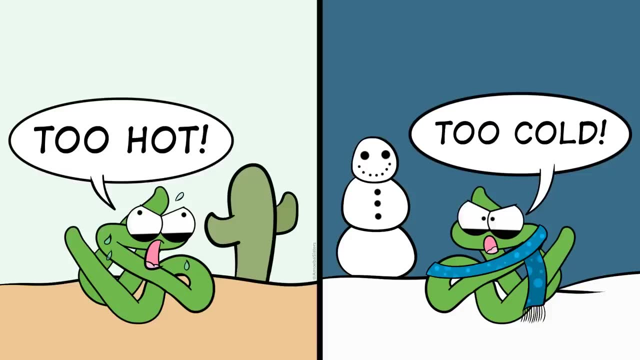 Check out some of our further reading suggestions in the description about that. One last thing we haven't mentioned. Each protein has an ideal environment for functioning, which might include a certain temperature or pH range. If the protein is exposed to something outside of its ideal temperature or pH range, it will.